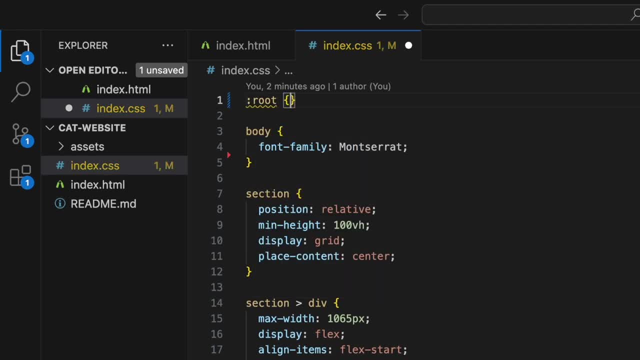 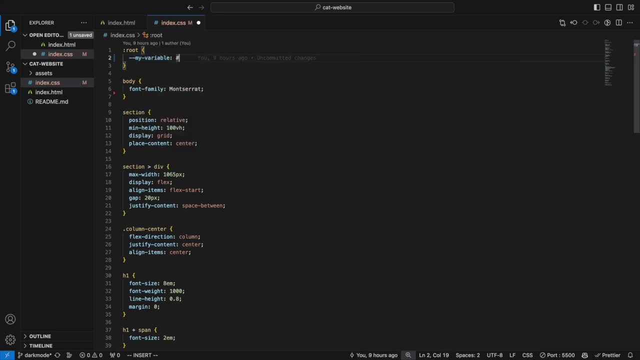 accessible anywhere and that's in the colon root. The variables in here gets something called a global scope. We can override these in the more specific places, like classes. Then they are locally scoped. But more on that later. Let's start by adding a text color variable for Light. 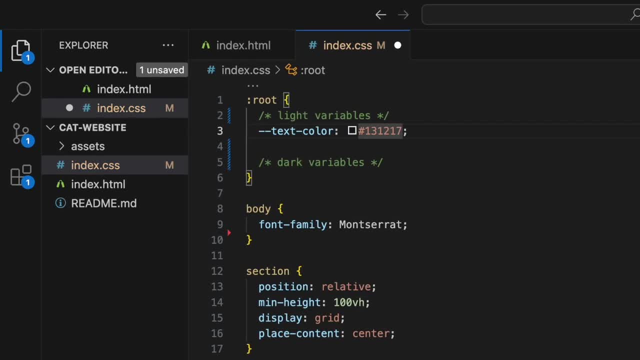 Mode and one for Dark Mode. We will also need a background color variable for both modes And, last but not least, we want to be able to change the button color. If you want to be able to change more things on your website, you can add as: 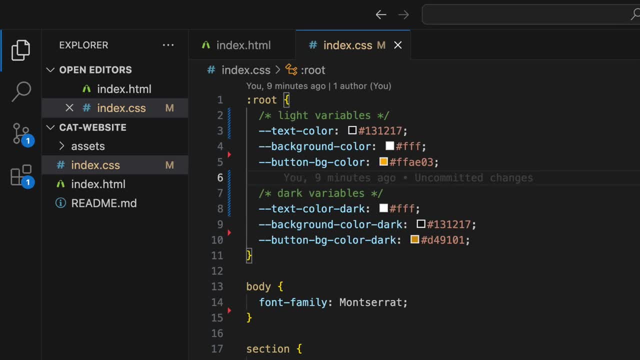 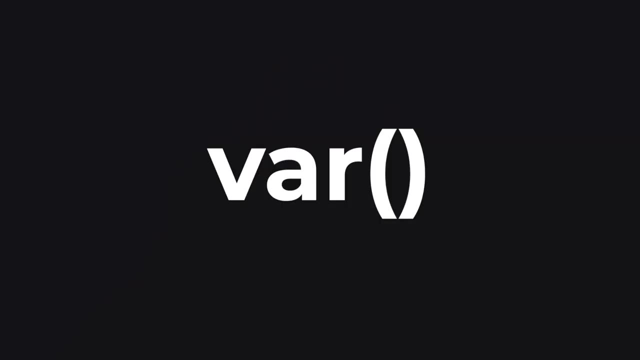 many variables as you want in here. Now you know how to create variables, But Chunky, You say, How on earth do we use them? That's a great question, my friend. Let me tell you about the var function. So CSS has a bunch of built-in functions. This is one of them. You can 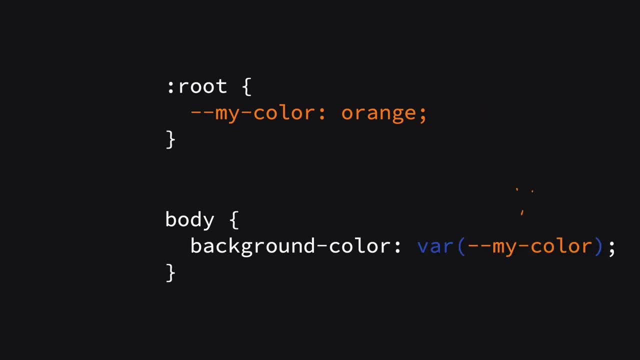 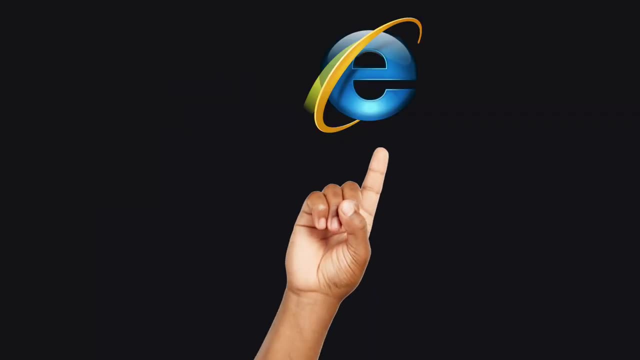 change the size of a property and put var with the variable you want to use inside. You also have the possibility to put a fallback value in the function. if you're targeting older browsers that might not have the support of CSS variables, But all the modern browsers support this CSS function. 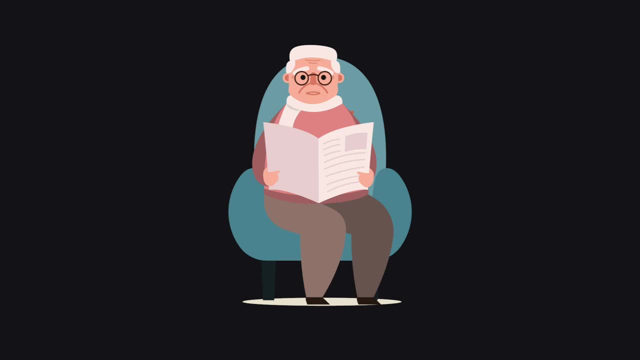 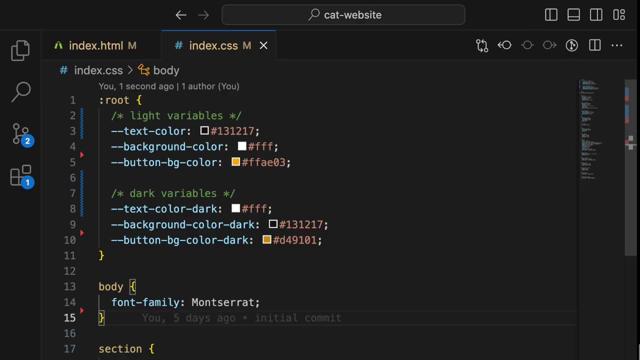 Now we know about CSS variables, So let's apply this newfound knowledge to add Dark Mode to our website. We have this good looking website here. I know it's amazing. We added the variables in our root tag earlier for Light Mode and Dark Mode. Let's put the 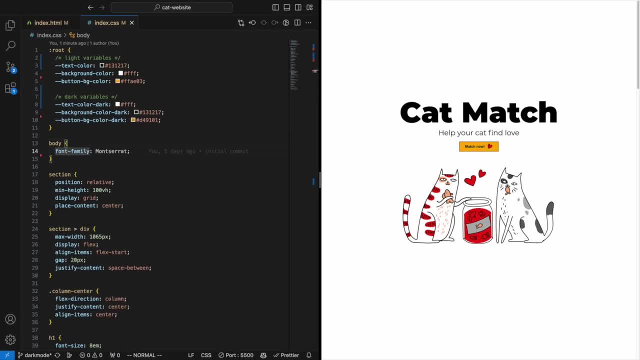 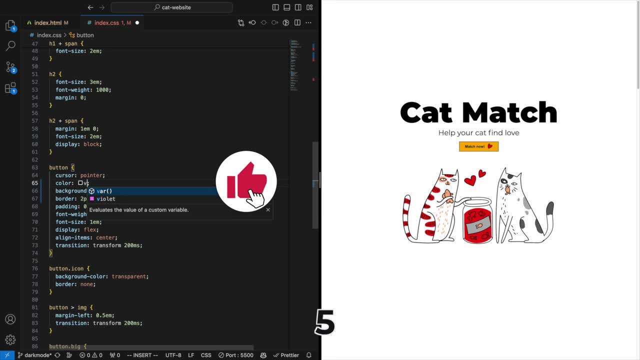 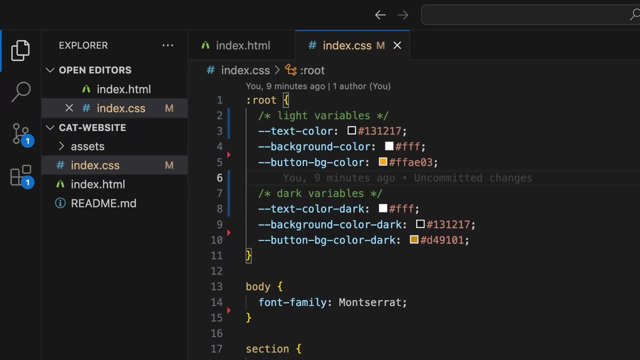 var function to use and set all our content to the light mode variables. I will tell you why in a minute. Oh, and please leave a like if you enjoyed the content. Awesome. Remember how I told you earlier about the global scope, where all variables in colon. 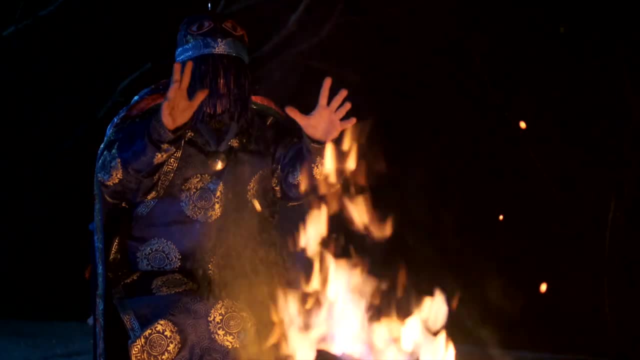 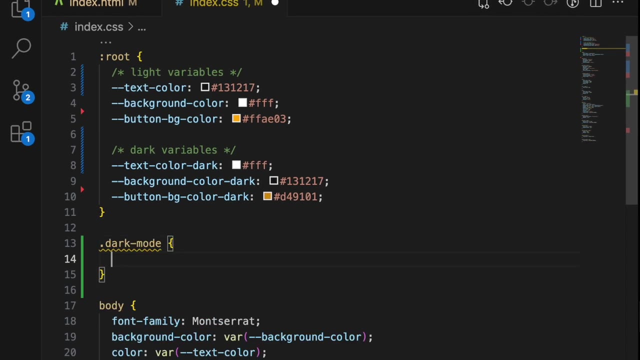 root would be accessible everywhere. Well, now it's time to apply some magic. using the local scope, We create a class called Dark Mode. Inside this class, you can overwrite the light mode variables with the dark mode variables. Now, if we add this class to the body tag in our HTML, we can change between light mode and dark mode.